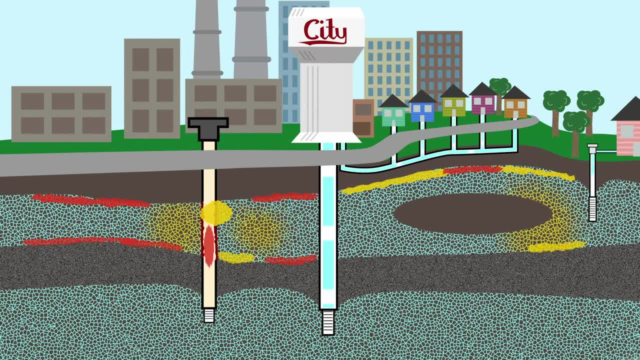 break down. pollution in shallow aquifers can travel into deeper groundwater supplies that would have been protected. When we pump water from our wells, it creates suction like a vacuum cleaner. This can pull nearby pollution into the well or down into a deeper aquifer City wells. 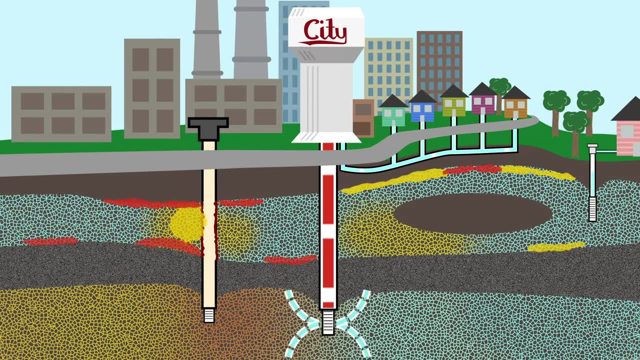 can pull pollution from farther away because they pump a large amount of water. Groundwater contamination is difficult to track and often goes unnoticed, especially in private wells that don't undergo the same thorough testing as city wells. If contamination is discovered in a well, the water should be pumped and treated until it is safe to 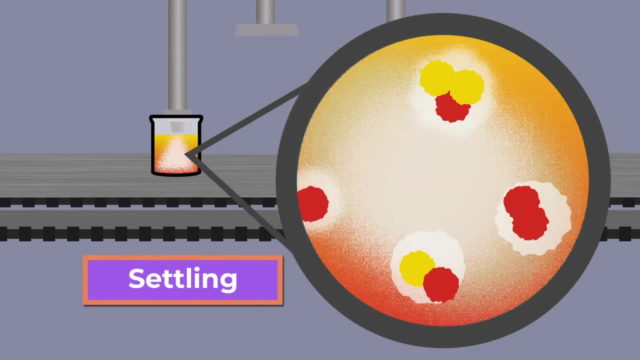 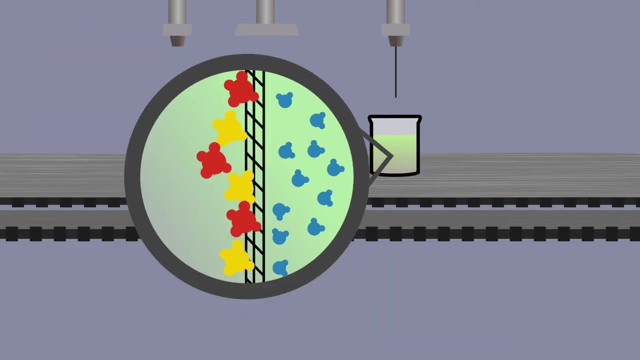 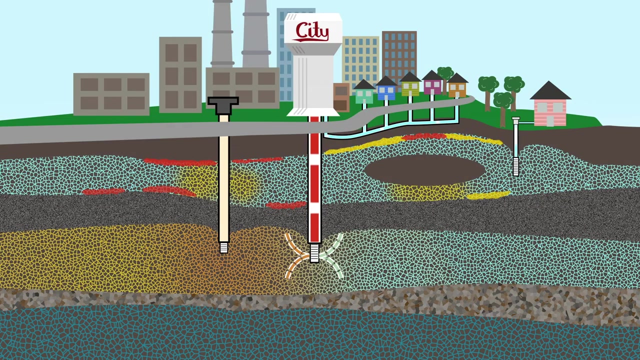 drink. The treatment process is complicated. It's complicated, expensive and depletes groundwater resources. Treating contaminated groundwater can cost ten times as much as preventing contamination in the first place. Other options to address well water contamination include drilling a new well or diluting contaminated 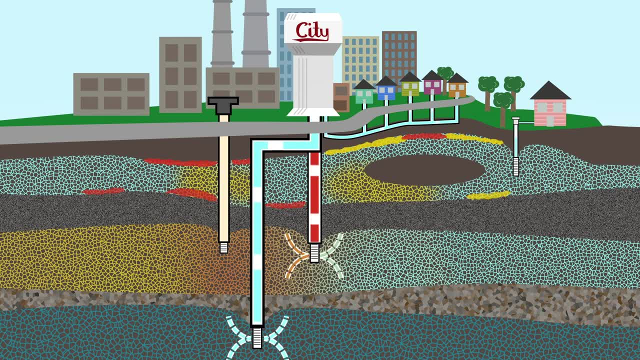 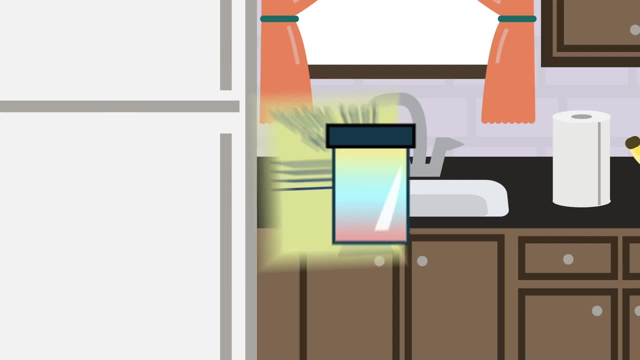 water with clean water. Regardless of the approach, your city will act to ensure the water you drink is safe. If you have a private well, you should test your water yearly for contamination. This is especially important if infants, the elderly or people with health conditions. 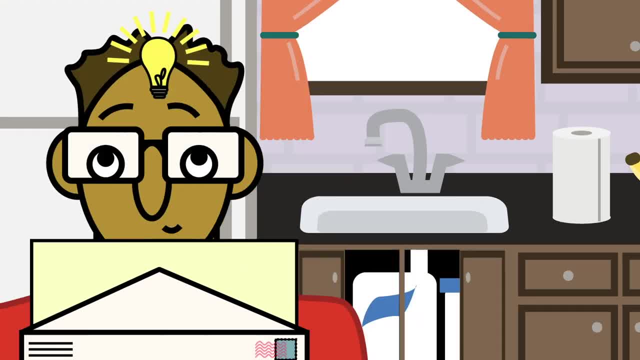 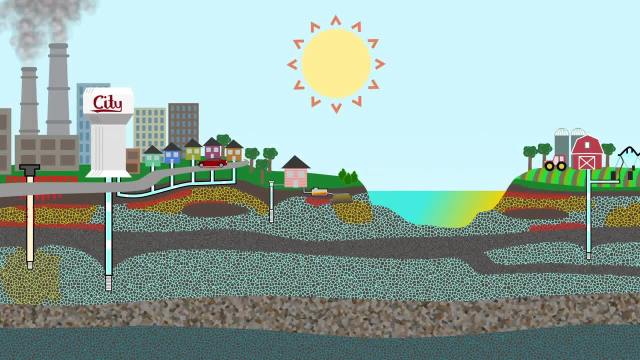 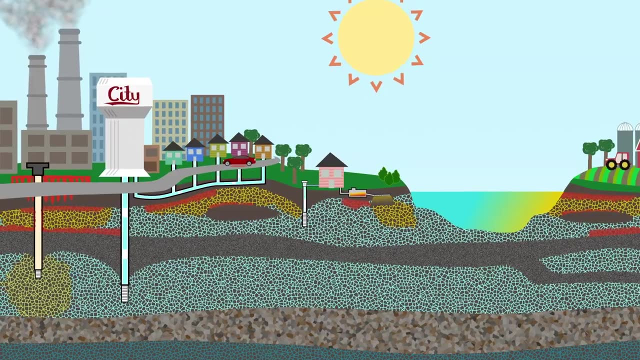 drink your water If contaminated. a home water treatment system can usually remove most pollutants. However, because treatment is so expensive, it's better for everyone if we prevent pollution in the first place. Whether you have a private well or are on city water, everyone has a. 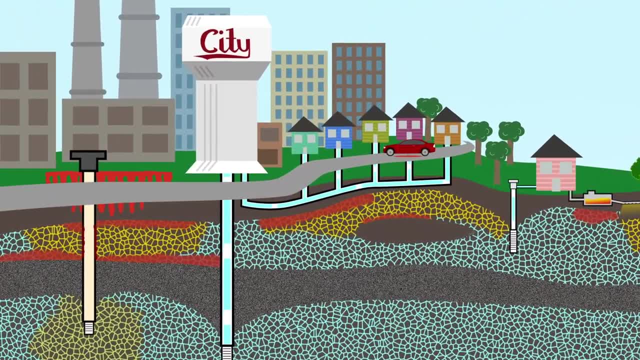 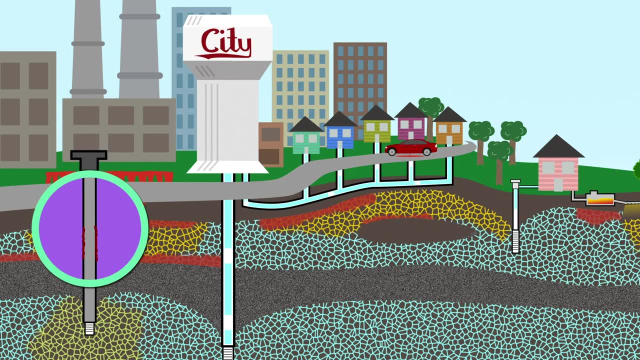 role to play in preventing contamination from getting into our groundwater. If you have a well that you no longer use, it is important to keep the water you drink safe. This has use. it is important to have it sealed by a licensed contractor with a special concrete. 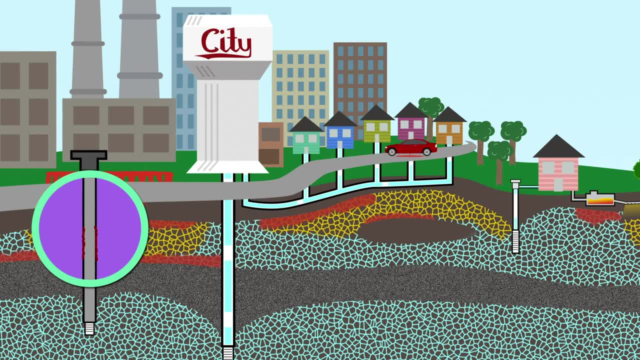 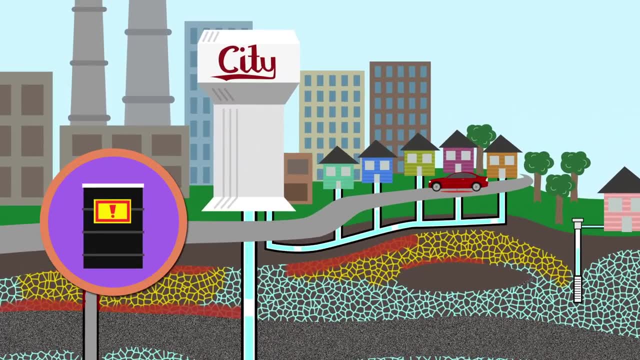 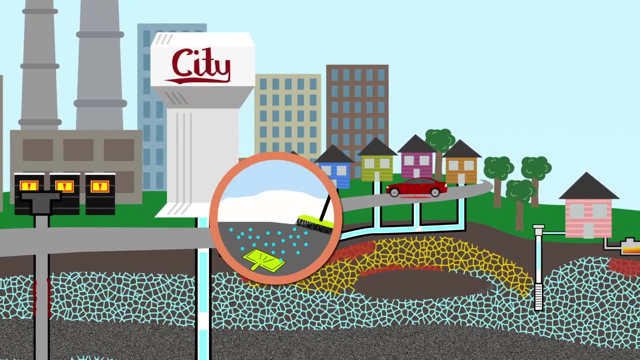 mix so it doesn't become a pathway for pollution. Property owners are responsible if contamination occurs due to their unsealed well At work and home. we can be careful to properly handle and dispose of hazardous waste. use environmentally friendly household cleaners, sweep up and reuse excess deicing salt and. 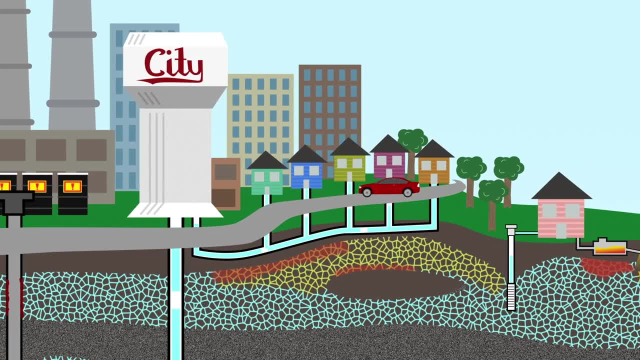 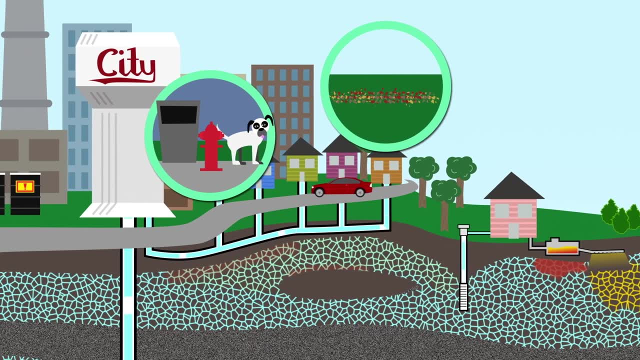 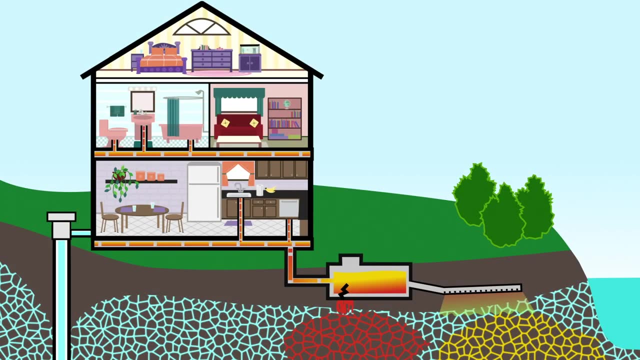 keep vehicles well maintained. Even small everyday actions go a long way, like picking up after pets, mulch, mowing leaves and grass clippings to reduce fertilizer use, and hand pulling weeds instead of using weed killer. Always be careful about what gets flushed down the drain.